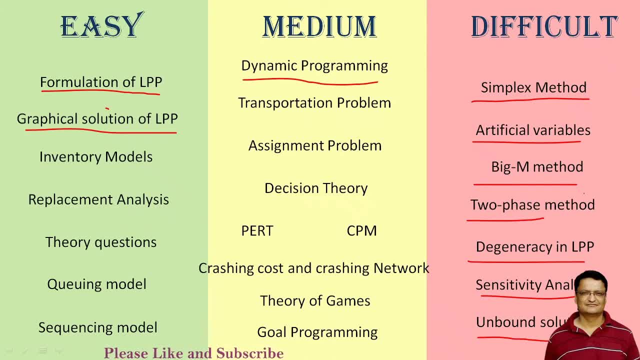 analysis in LPP and unbounded solutions. These are the only things which are little difficult, But don't worry about that. You can concentrate more on this easy section and this medium section. Now, inventory control is a very, very easy stuff. You can start with replacement. 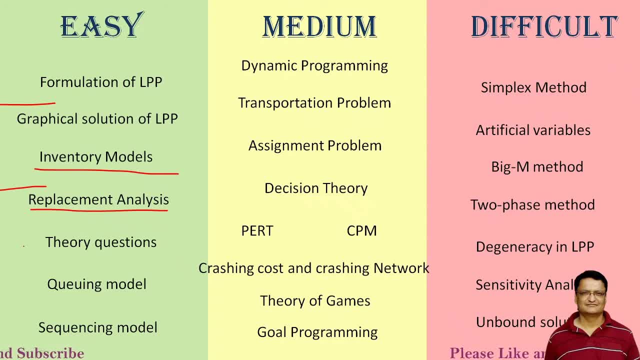 analysis. You can start with the theory of theory questions. like so many university papers have some theory questions and you can opt for those, But I will recommend that, instead of theory questions, focus on the numericals, because they will guaranteedly give you a maximum marks. Theory- 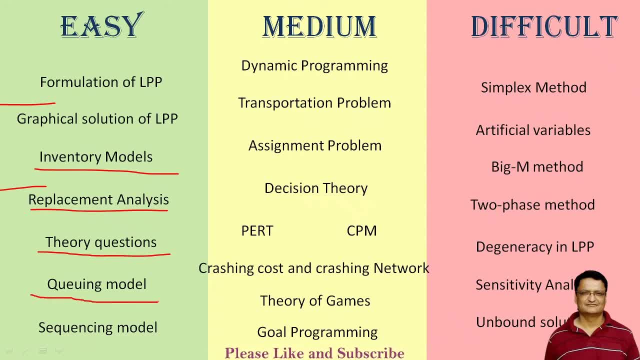 questions may give you some average marks. Then, queuing model: a very simple: you need to remember few formulas and you can score the out of marks. Sequencing model: a very, very easy thing to go for. Now the transportation problems: Yeah, so they are quite an easy one and you can go for them. Now there are various problems. 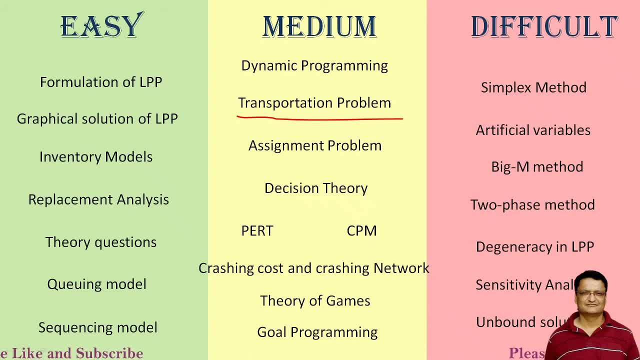 Variety of problems are there and all of them are quite easy. Assignment problems: Yes, you can go for decision theory- Again, it is very easy. Power and CPM: Yeah, so it will be more of an easy and medium level right, Then crashing. 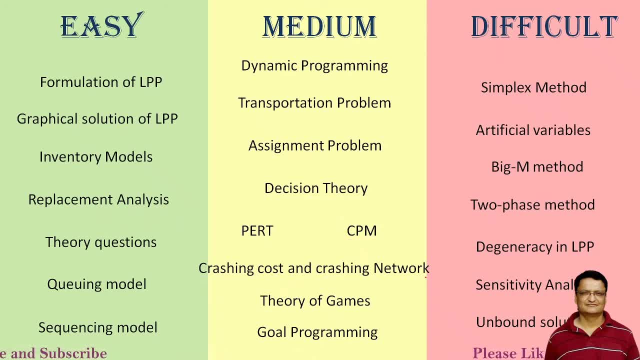 Cost and crashing network is also point of. in very easy topics- Theory of games- Some four, five technique can work, formulas and goal programming. So what? I will recommend that you discover all this easy part week that is applicable to you. Try to cover this. 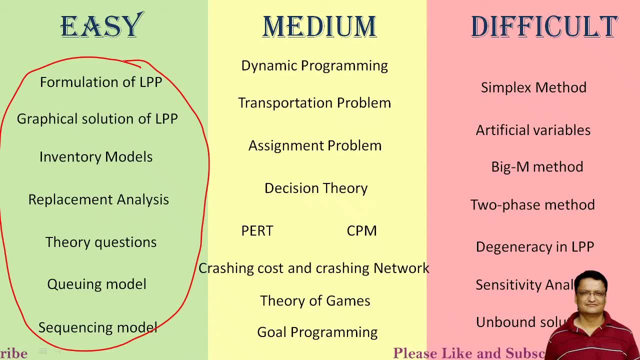 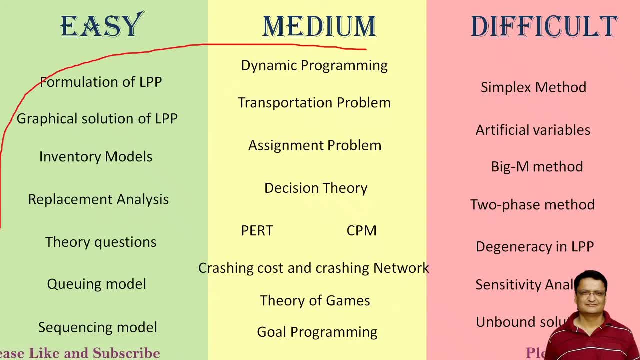 If you're looking for just getting pass, right, so these two section will give you more than 60% of marks, and if we really looking to score the war, then you can go for this difficult section now. how to study for this, right? okay, so how to study for this.